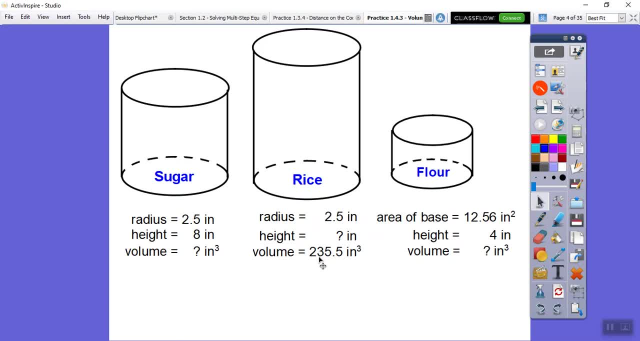 And we're looking for the height, but they give us the volume. on this guy, on this one, they give us the area of the base, that's the pi r squared, is the area of this circle right here. And then here's the height and we're going to look for the volume. Okay, and notice, volumes are always in cubic units, in this case inches. so inches, cubed or cubic inches, Okay, and then the dimensions are always in in singular units, or just inches, Okay, so so an area, you see this. 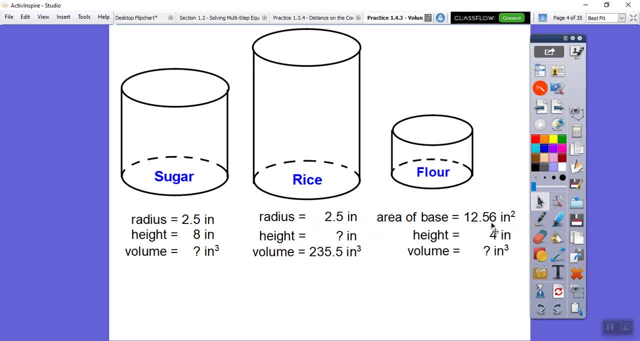 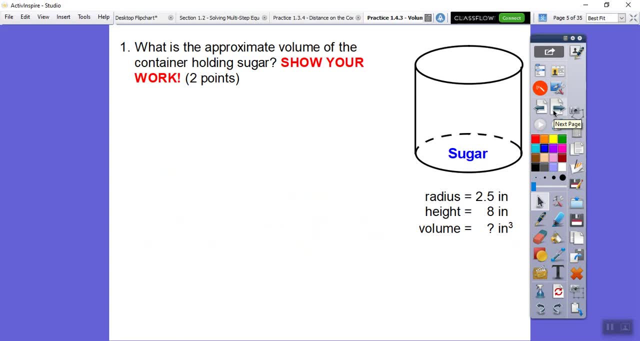 area area is always inches squared. So let's, let's do some of this, So let's go ahead and let's find the approximate volume of this container that's holding sugar. Okay, so this is the first one right here. So the volume of a cylinder and of a prism- I don't know if you've done prisms yet, but same with the prism- is base times, height, and B is the area of the base And since it's a circle, the area. so here's the area of the base, right here. 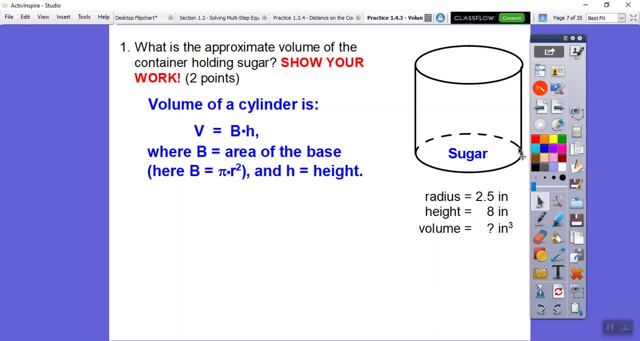 Here is pi, r squared and then times the height. Okay, so we know the r. we're going to square that. multiply it times pi, which is 3.14 times the height, And then that's going to be our answer in cubic inches. Okay, so let's go ahead and plug that in. Okay, 3.14 goes here And then 2.5 goes here. I'm going to square that. you got to do the exponent first, So before we can multiply, we must square this first. order of operation says exponents come. 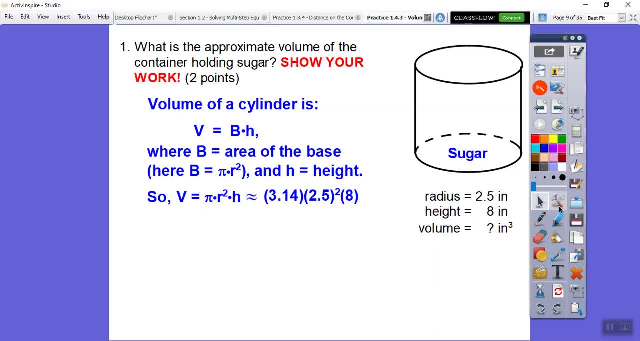 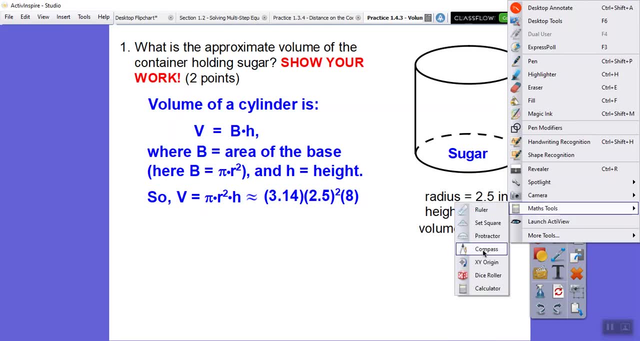 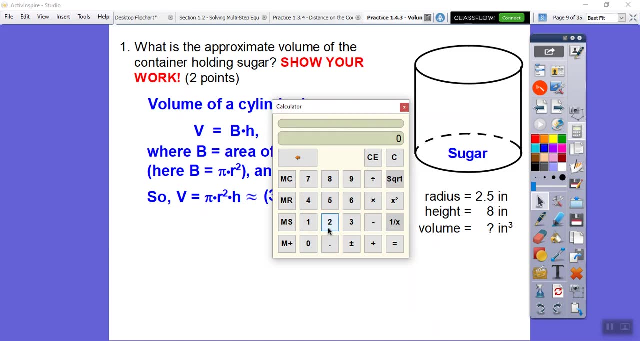 before multiplying. So I'm going to do 2.5 times 2.5. And I think I can show you on this calculator there's. there's all kinds of calculators in here, So there might be some teachers coming in. you might hear some stuff on here in my classroom early in the morning. So 2.5, you can just do 2.5 times 2.5. Or you can hit this squared button. This is this one square root. I'm sure I'm positive your calculator looks a little bit different, But I'm 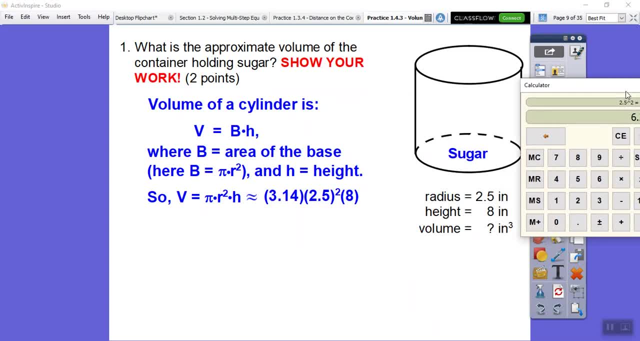 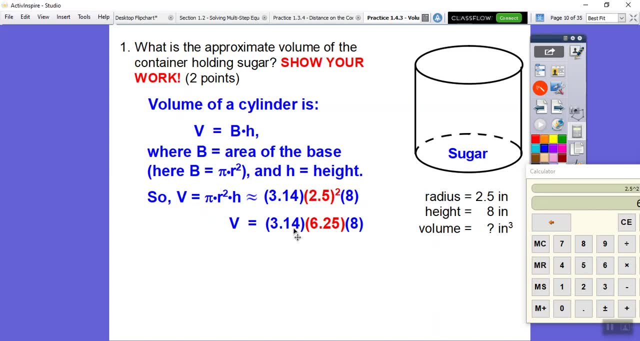 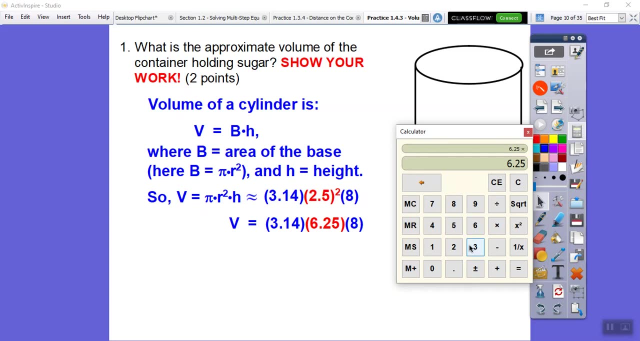 just going to square that, And so that's going to be 6.25.. So let me just move the calculator out of the way. So there's, this is right here. this is 6.25.. And then we just multiply times 3.14, times eight, and then that's going to be our volume. So we still have 6.25 in there. So I'm going to go times 3.14, and then times eight, And then that's going to give us the volume in cubic inches, So it's 157.. Okay, so 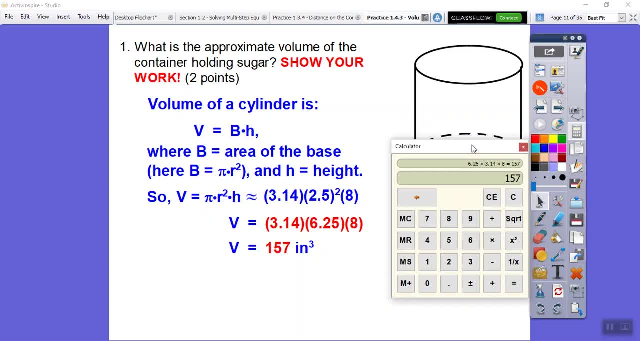 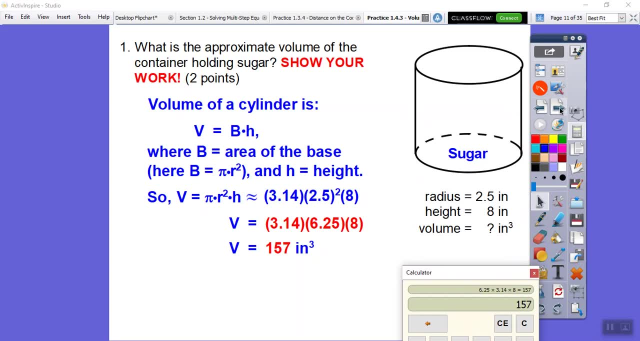 so here it is right there. So the volume is 157 cubic inches. that's the volume like if I wanted to fill this whole thing up with sugar. that that's how much volume it has in there to hold all the sugar on there. Okay, so let's, let's use that same formula here to find the approximate. 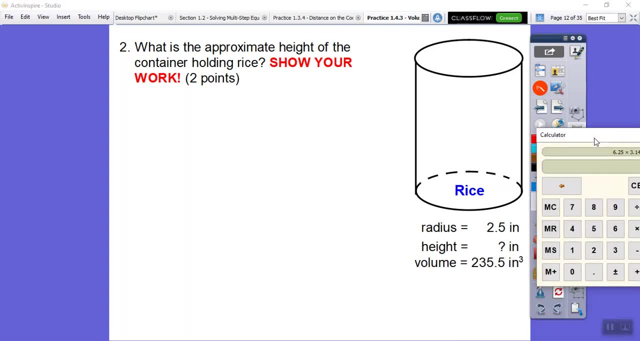 height of the container that has rice. Okay, so here, here's the volume. this is my V. So this equals pi times this squared times h. Okay, so we're going to plug all that in, So let's go ahead and do that. Okay, so volume equals base times height. So the volume is two point or 235.5.. So 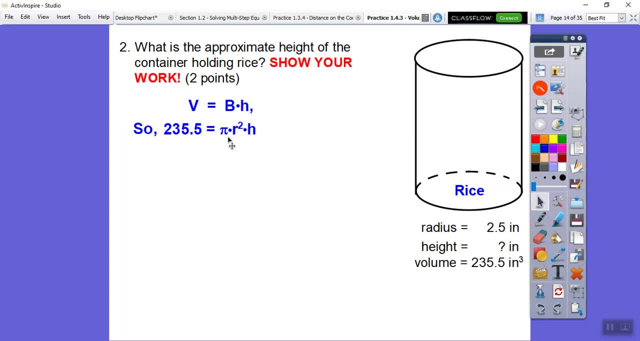 that goes here in the volume position: 3.14, 2.5.. And we have to square that first and then we'll divide it out to get h. Okay, All right, so 2.5 squared, remember that's 6.25.. And then 6.25. 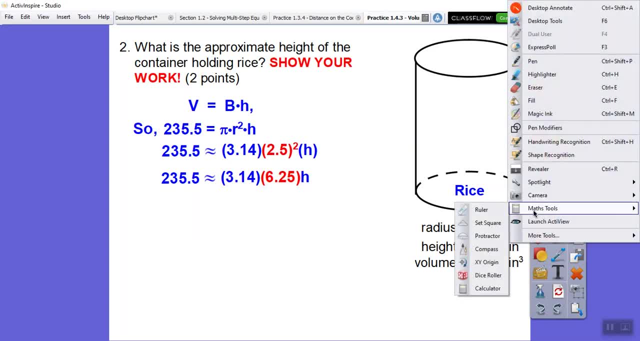 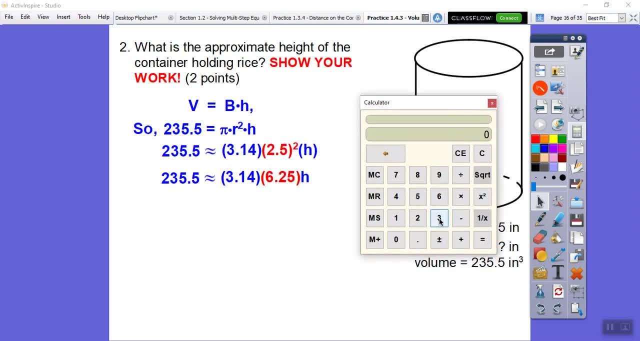 times 3.14.. Again, I'm just going to pick up my calculator And I have the answer here, But I just want to you guys. I have students. I say, use your calculator. they just don't want to use it. So let's go ahead and use this: 3.14 times 6.25.. Oops, I did times 6.25.. 6.25 equals okay. 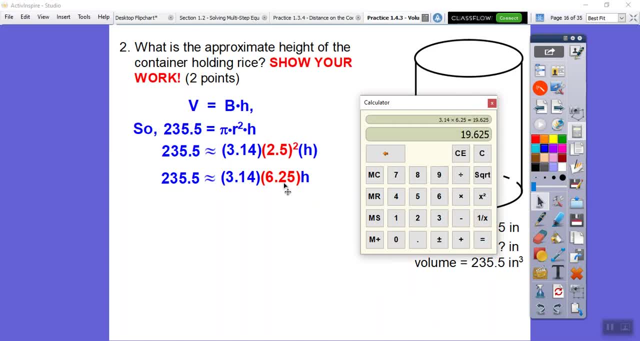 so 19.625.. So it's going to be: 19.625 times h equals this 235.5.. Okay, now this says 19.625 times h. so we have to do the opposite of times and divide. So I'm going to divide both sides by this 19.625.. 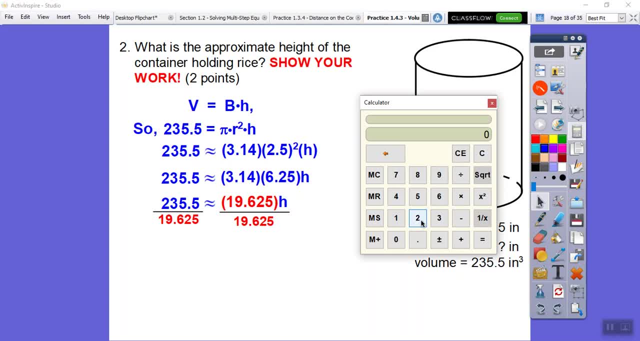 So 235.5 divided by 19.625,, 235.5 divided by 19.625, and that's going to get me 12.. Okay, so the height is 12 inches. Okay, so let's go ahead and plug that in. 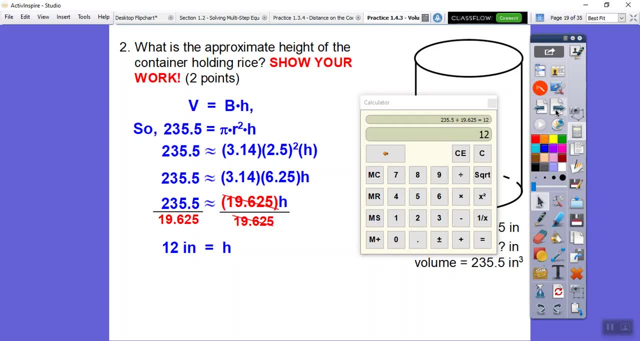 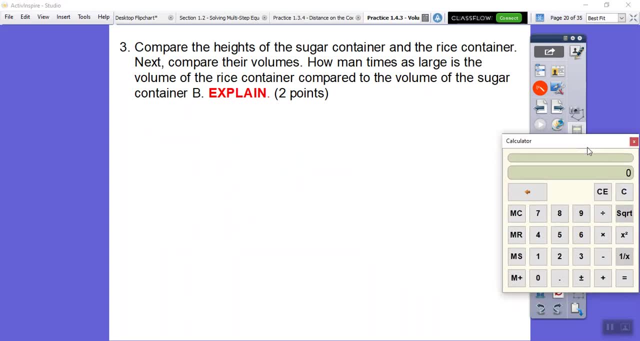 Okay, all right, so let's answer some more. So there's that guy right there, All right. so this guy says to compare- I'll just move this away- So compare the heights of the sugar container and the rice container, Okay, and then we're going to compare their volumes. 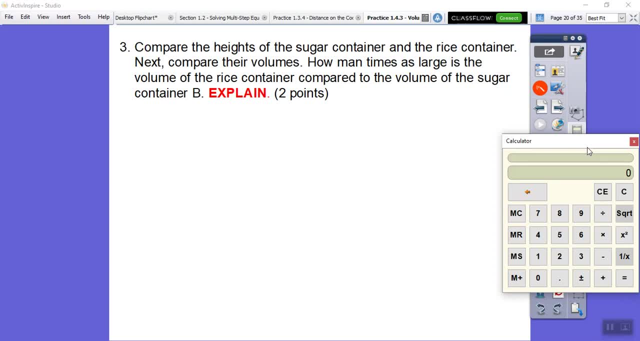 How many times as large is the volume of the rice container compared to the volume of the sugar container? Okay, I know, because I teach math. It's kind of hard to see if you don't know. But they want us to compare the heights. 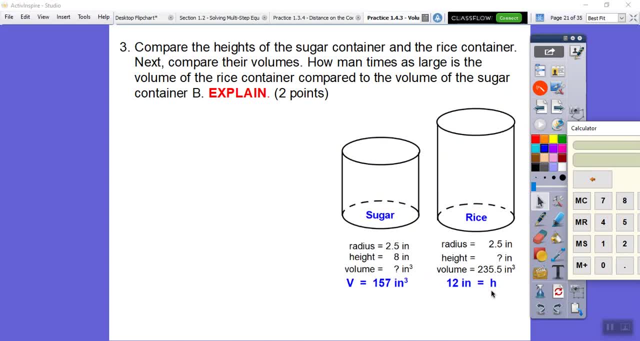 Notice, this height is 8, and this height was 12. right here The volume of the sugar was 157. And the volume here is 235.5.. So the sugar height is 8 inches and the rice height is 12 inches. 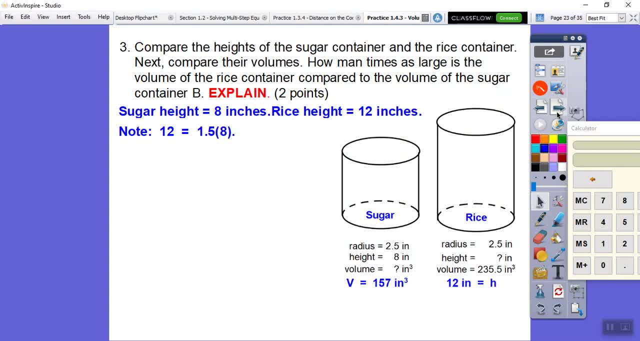 You probably don't see this, but 12 happens to be 1.5 times 8. And so this is really hard to see. So the height of the rice is 1.5 times the height of the sugar. I'm not sure what they're asking for, but if I was teaching this, I would want you to recognize that. 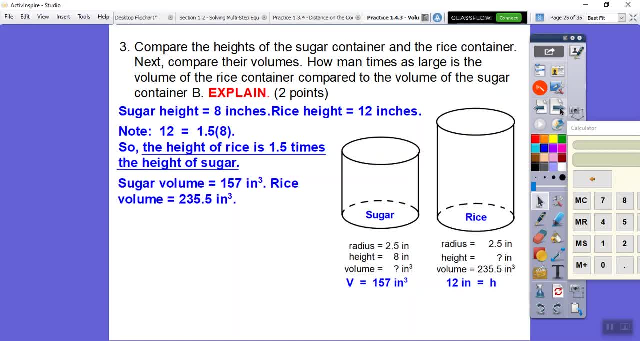 Okay, So then we're going to do the same thing with the volumes And let's just see what kind of relationship they have. Okay, Is this 2.5 times this? So I'm going to. I'm sorry, did I say 2.5?? 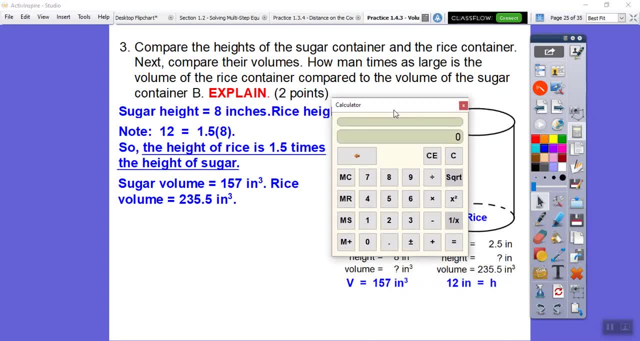 1.5 times this. Let's multiply 157 times 1.5.. Let's see if we get that, And if we do, then we're going to state that So 157 times. oops, I didn't mean to do that. 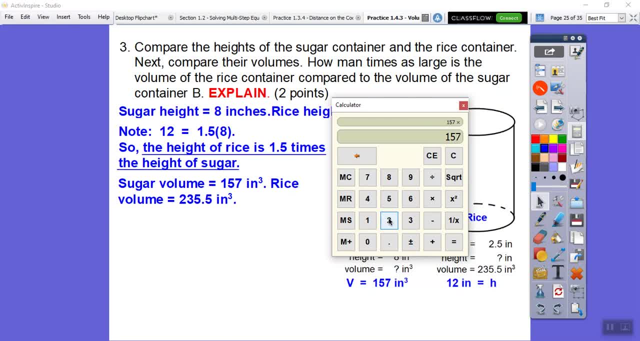 157,- it's hard as I'm doing it like here- times 1.5.. 1.5 equals- hey, what do you know? 235.5.. So let's go ahead and conclude that right there. that the volume. 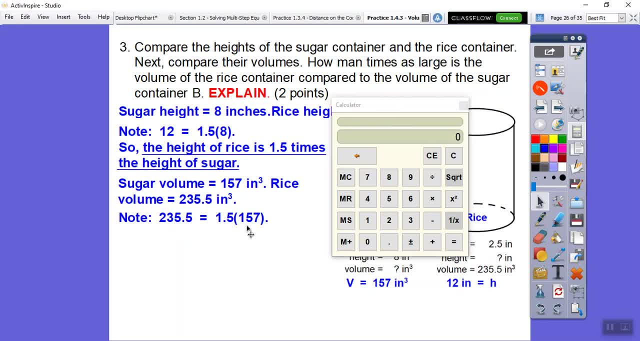 of the bigger container happens to be 1.5 times the volume of the smaller container. And notice up here the height of the bigger guy is 1.5 times the height of the smaller guy. Notice they both have the same radius. 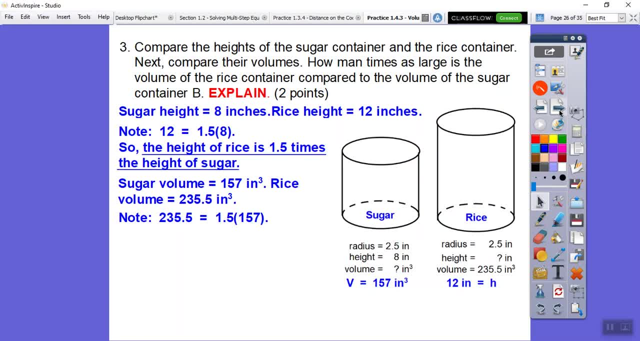 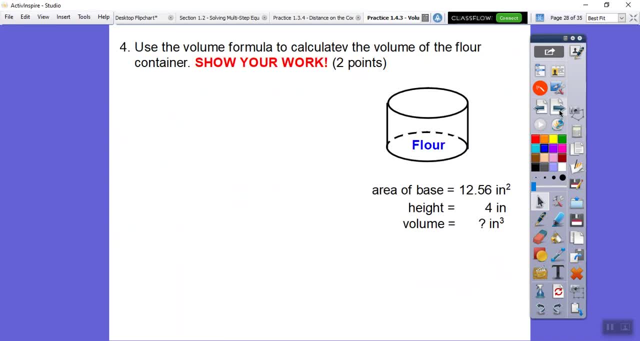 So whatever height this guy increases, so does the volume, As long as they have the same radius. So the volume of the rice is also 1.5 times the volume of the sugar. Okay, So here I'm sorry, I went too fast. 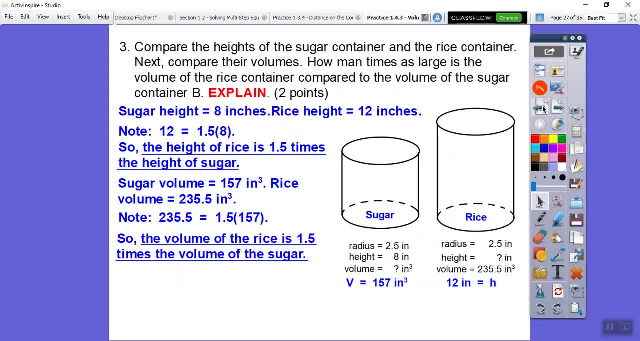 Let me just do that And you can just pause it whenever you need to, you guys. So some people say I go too fast And I don't know. I'm teaching and I'm trying to supplement some teachers here. So anyways, if you need to, please watch it a second time or rewind it a little bit. 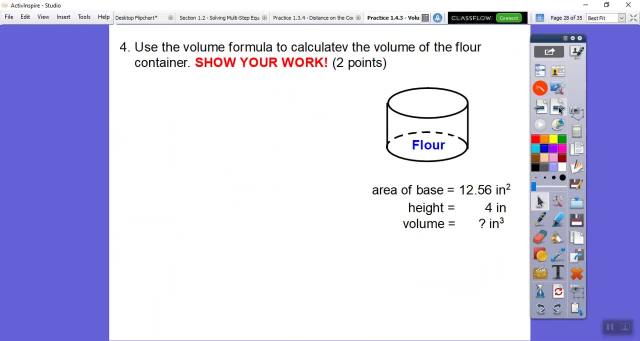 And if you didn't hear it, you guys at least have that. So all right. So we're going to use the volume formula here to calculate that there shouldn't be a V there to calculate the volume of the container. Okay, So the area of the base is 12.56 square inches. 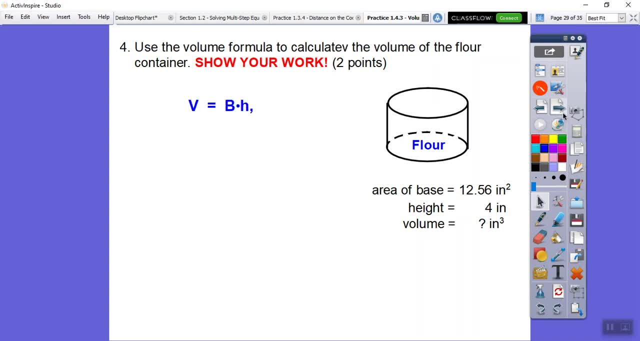 And so we know the height and we know that we're looking for the volume. So remember, volume equals base times height. Here's the base right here: 12.56.. Here's the height times four. So we're just going to multiply those. 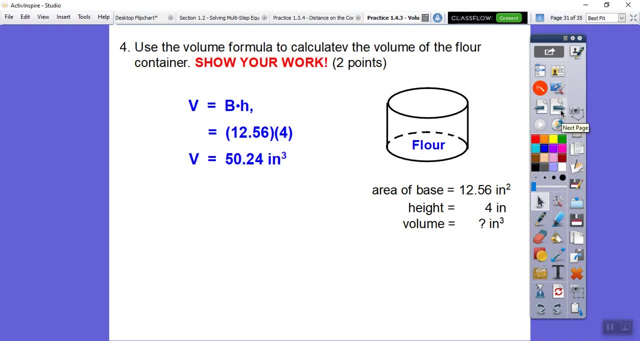 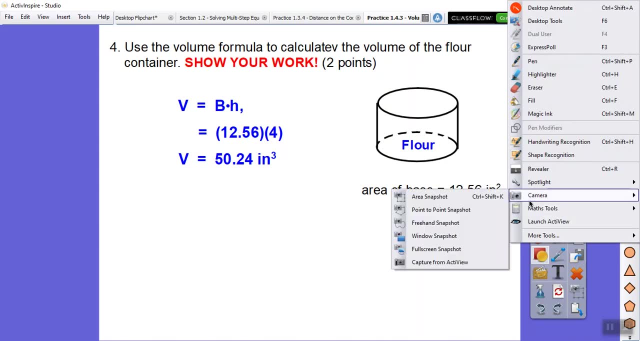 So those give us 50.24 cubic inches. When we do that 12.56 times four. Let me do that. Sorry, you guys, I'm sorry, 12.56 times four. I'm trying to hurry because I got students coming in soon. 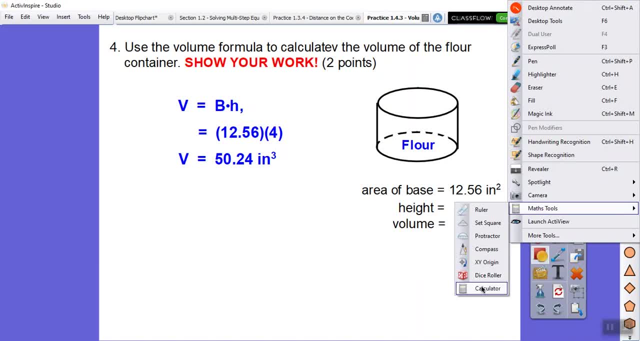 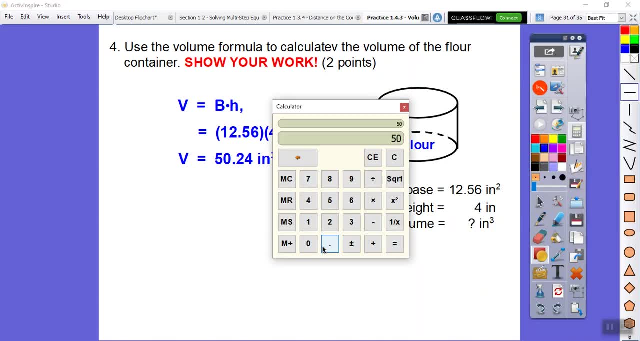 And I tried doing this last night and my wife came home And it's just, it's hard for me to record these things. What am I looking for? Calculator- Sorry, Hard to talk and think at the same time too. 50.24 times, what was it? 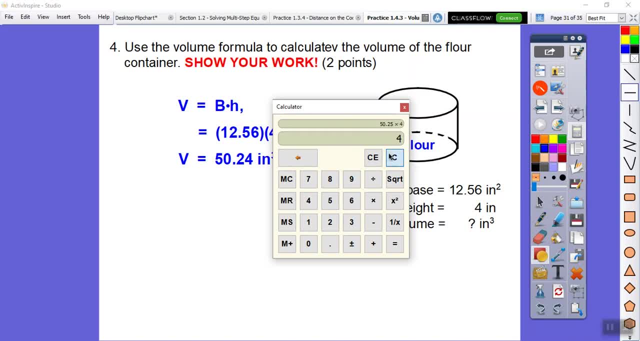 Times the height over here, Four times- oops, I did it backwards, Sorry- 12.56.. Not bad Times. the height of four. That's where we get that 50.24.. So remember volume is always cubic inches or cubic units. 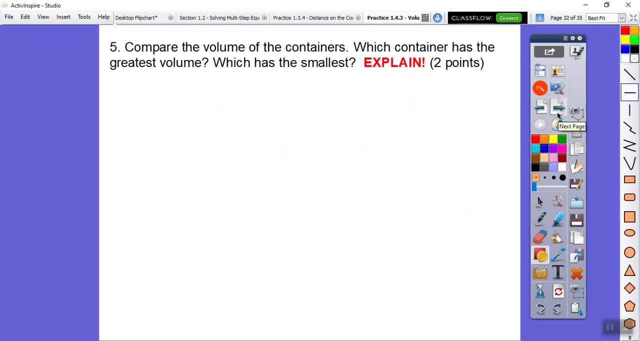 Okay, All right, we've got a couple more. So compare the volumes of the containers. Which container has the greatest volume, Which one has the least? So here's our containers right here. So here's the volume. The volume of this guy is 157..